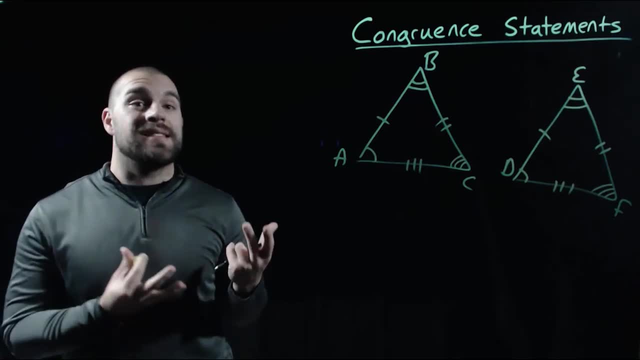 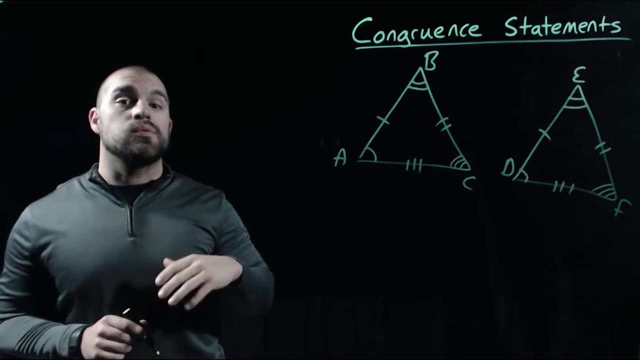 They've got all the same size sides. So what we can do is we can write out a statement that says these two figures are congruent. Now, one thing we have to be careful about is when we write out our congruent statement, is we have to match up the congruent vertices or corners of our shape. 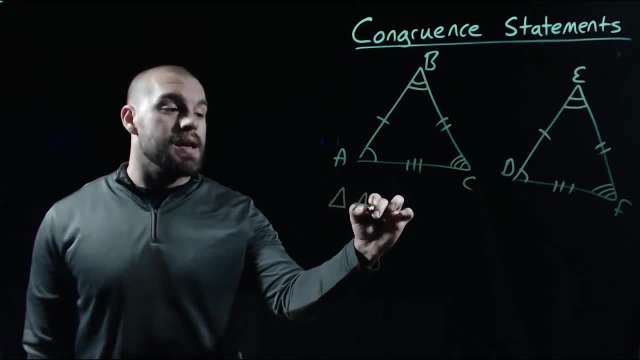 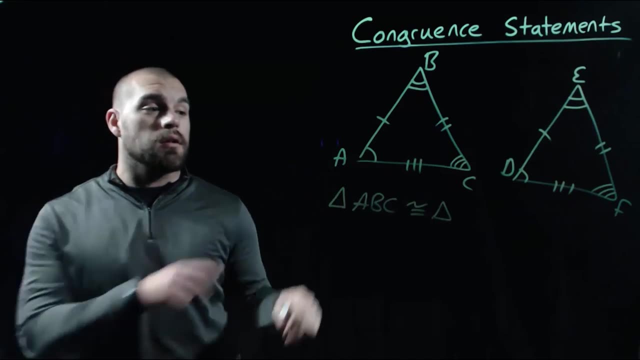 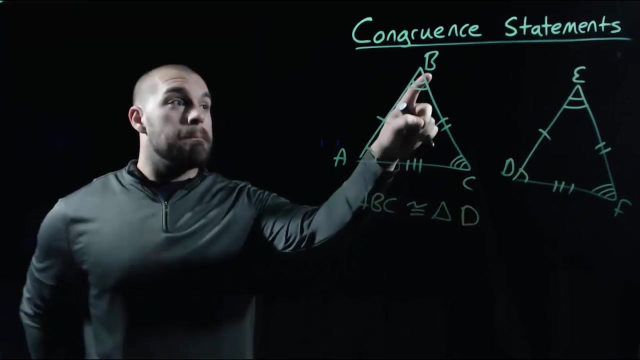 So if we decide to name our first triangle ABC, then what we have to do is we have to keep the same order when we're identifying the second triangle. Angle A is congruent to angle D and since we started with that started with, angle A will have to start with angle D. B is congruent to E and since B came, 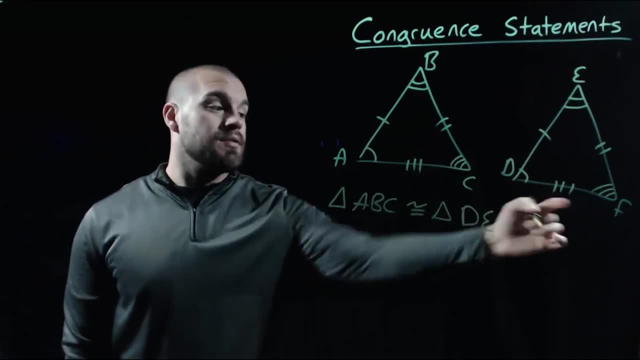 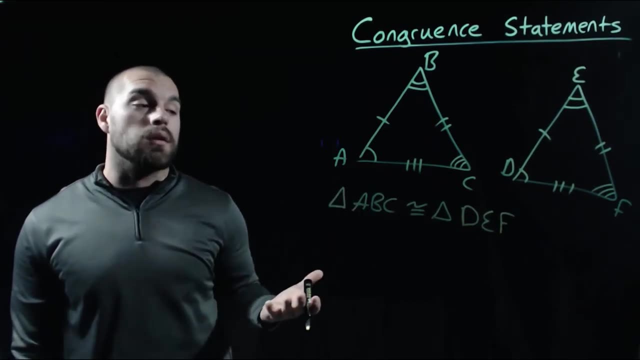 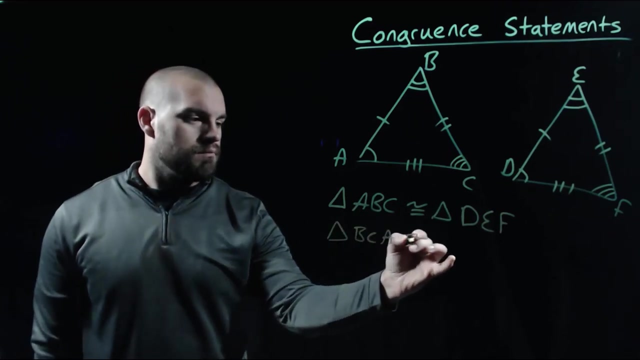 next. E will have to come next, and then angle C is congruent to angle F, So we have to call that second triangle DEF, based on how we named the first triangle. But this isn't the only congruent statement that we can write. We can change the order on these things. So let's say we called. 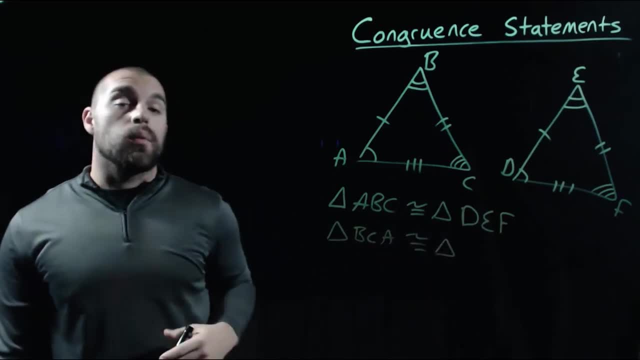 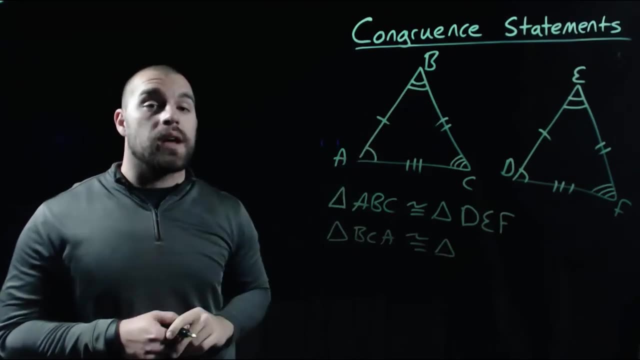 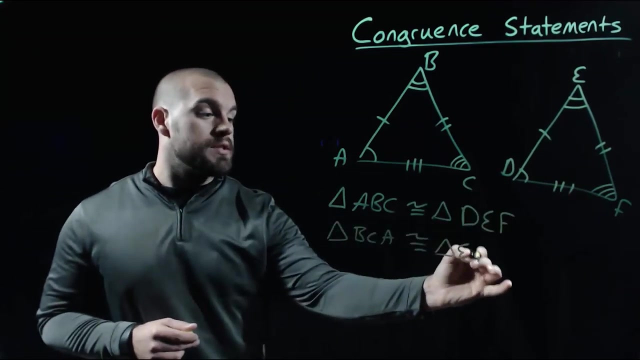 that first triangle, BCA, Then when we start naming our second triangle, we're going to have to adjust accordingly. Since we started with angle B, well, B is congruent to angle E, so when we write out this one, we're going to have to start with angle E. C came next, so F is its corresponding. 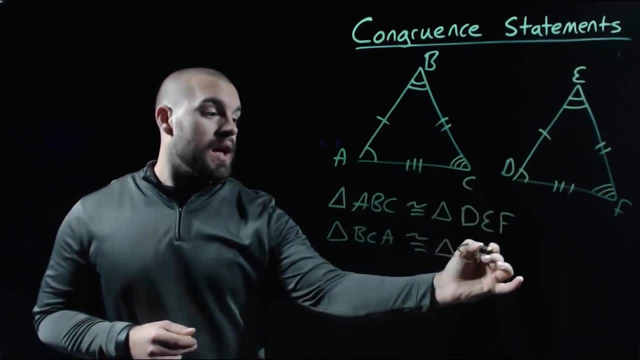 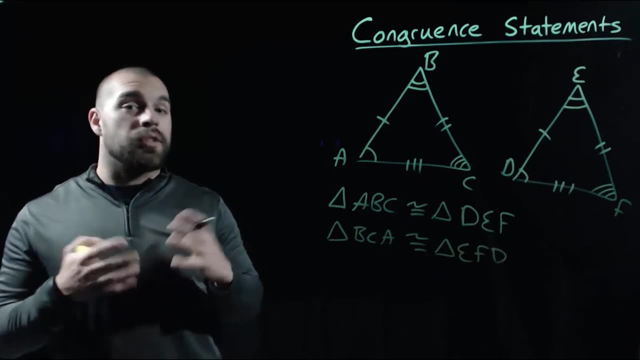 piece and then our last one was A, so we'll have to end with angle D. So the way we write the congruent statement doesn't really matter, as long as we match up the corresponding or congruent statement. So let's say we have a triangle B and we have to start with angle E. 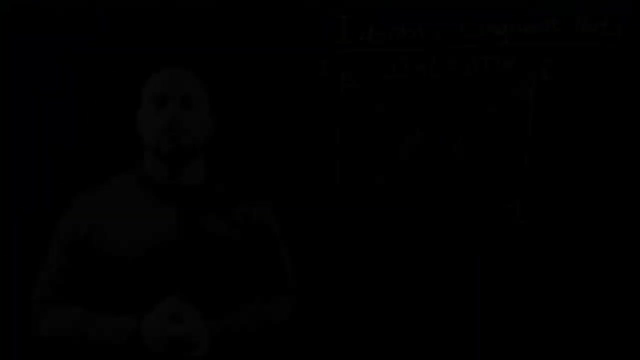 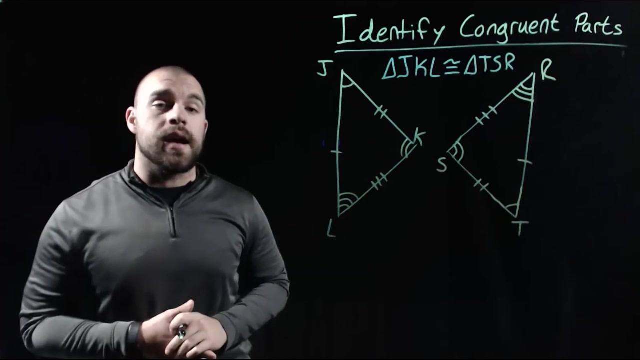 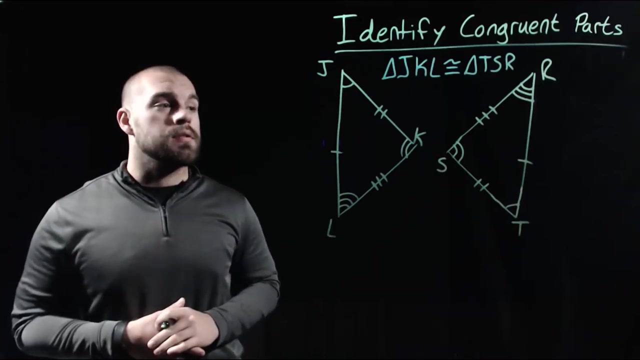 In this example, we're given two congruent triangles. We've got triangle JKL on the left and triangle TSR on the right-hand side. What we want to do is we want to go through and identify all of the different congruent pieces of these triangles. So let's start off with the angles. 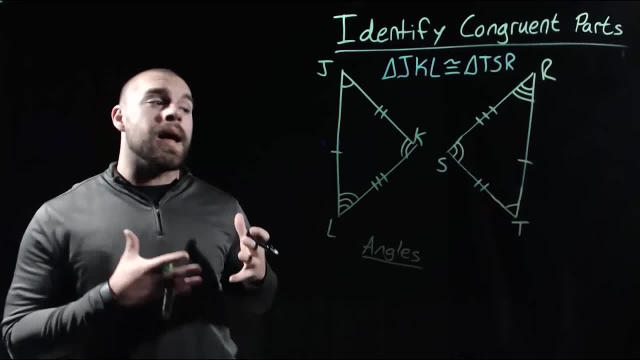 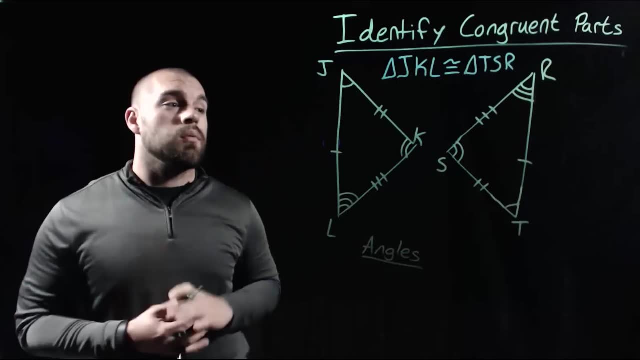 Now I think the easiest thing to do is going to be to look at the diagram and the markings that are given to us. We've got a bunch of arcs in the angles that show that those things are congruent. So if we start with this triangle on the left-hand side, let's 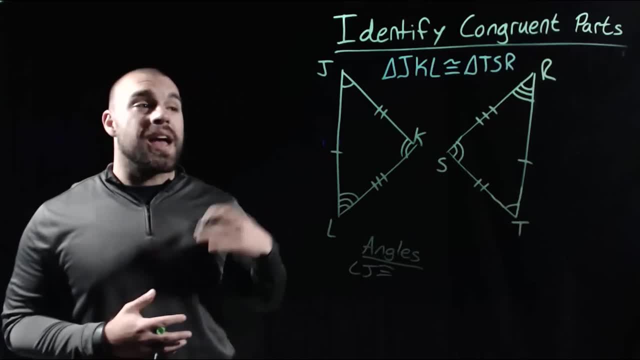 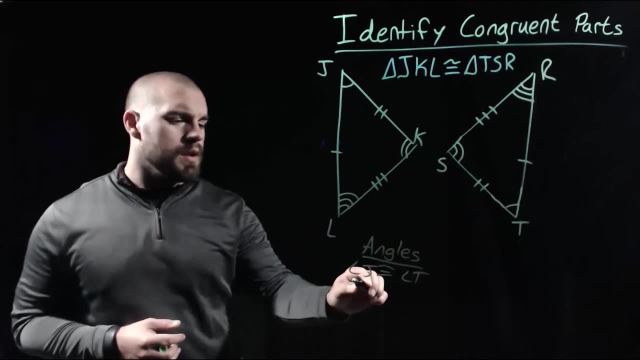 maybe look at angle J first. Angle J has one arc in it, so if we're looking at our other triangle, we need the one that also has one arc in it, So that's going to be angle T. Next let's look at angle K. K has two arcs in it, so if we're looking at our other triangle, 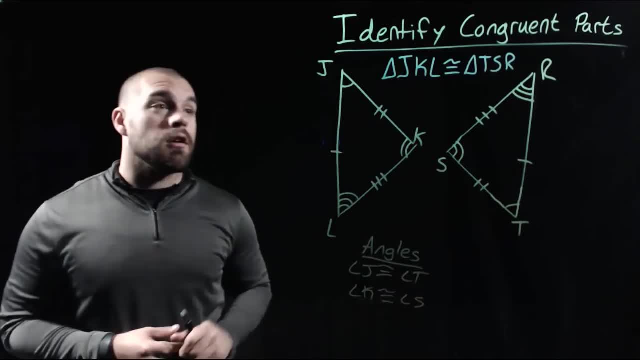 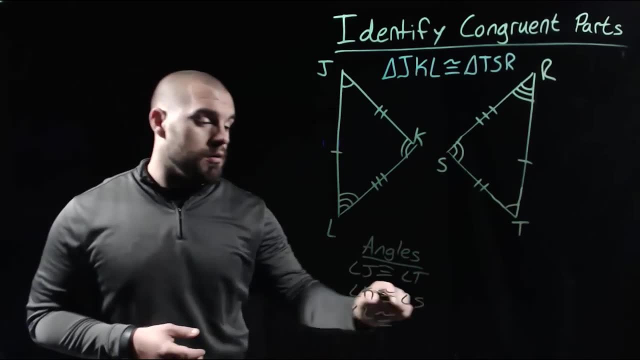 we need the one that also has two arcs in it, so that'd be angle S. And then our last angle from that first triangle is angle L, and the only angle we haven't used yet from the other one is angle R. So those are all of our congruent angles. Now, if we start looking at the congruent 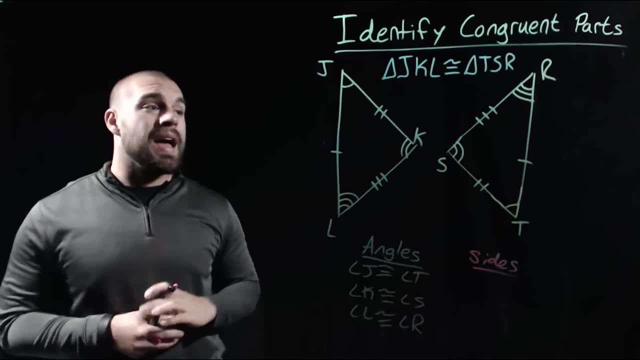 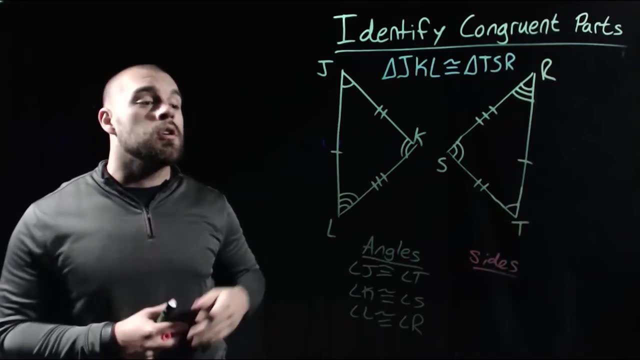 sides. we're also going to look at things that are marked out similarly. We've got dash marks on all of these sides, so we're going to look for the pieces that are congruent to each other or that are marked similarly. So if we start with JL on this left-hand triangle, 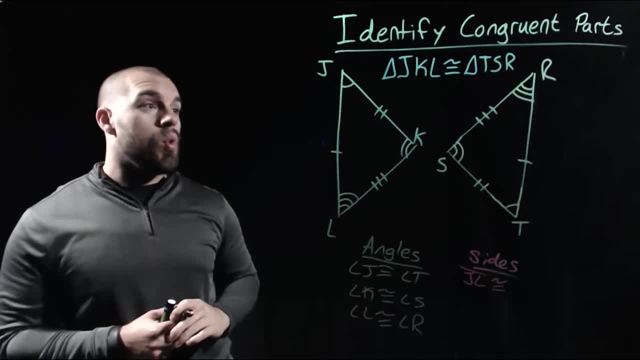 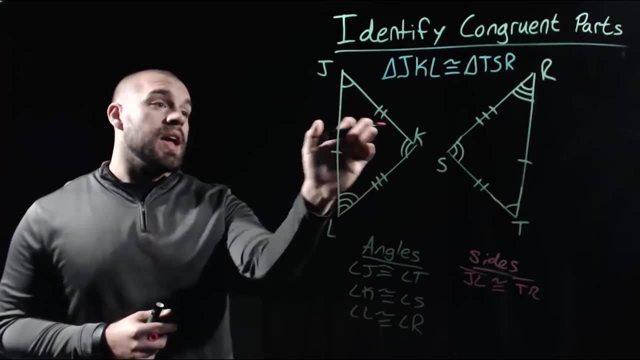 if we're looking at our other triangle, the one that has one dash mark on there, would be the segment that goes from T to R. Now, if we look at the segment that runs from J to K, that one has two dash marks on it. 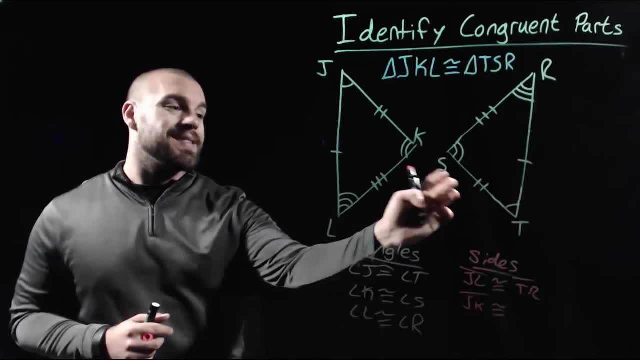 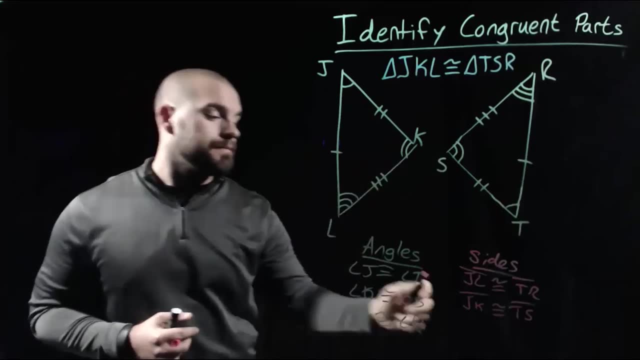 And if we check out our other triangle, this one that runs from T to S also has two dash marks on it, And then our last sides. we've got this piece that runs from K to L And matching up with that one, since that has three dash marks on it, we'd be looking at this side that runs from S to R. 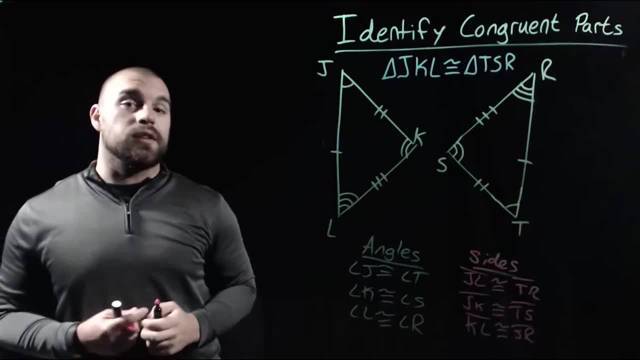 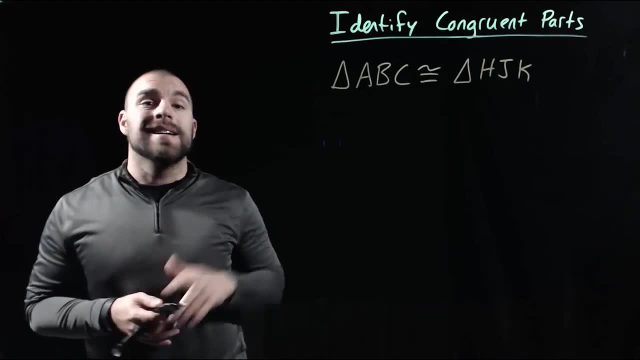 So there's all of the congruent angles and all of the congruent sides listed out. Now, when we're looking at identifying congruent parts, we're not always going to have a diagram to look at. Sometimes we've only got a congruent statement. So here we've got triangle. ABC is 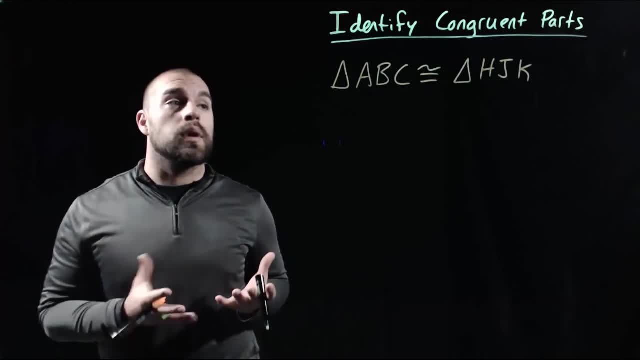 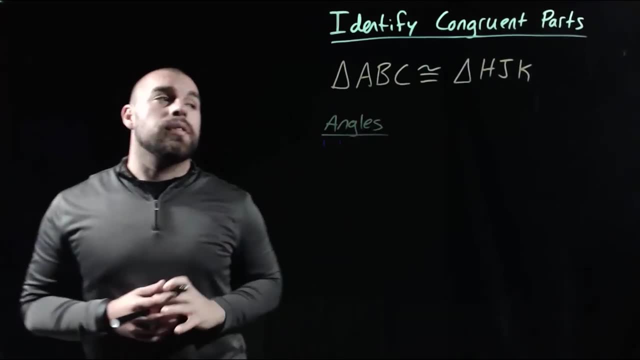 congruent to triangle HJK, And what we're going to do is we're going to go through and identify the congruent angles and the congruent sides. So let's start off with the angles. The nice thing about these congruent statements is that they're written with their corresponding 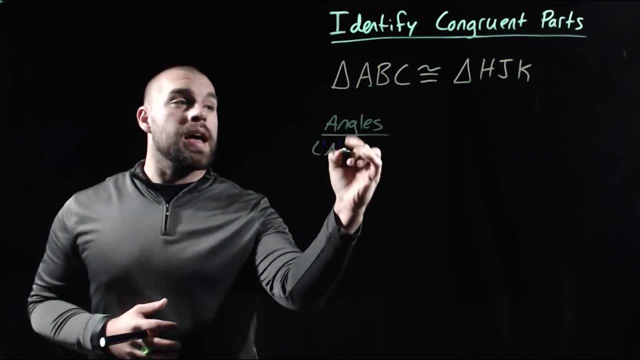 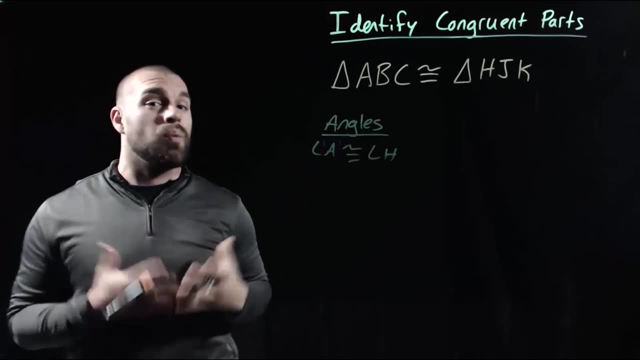 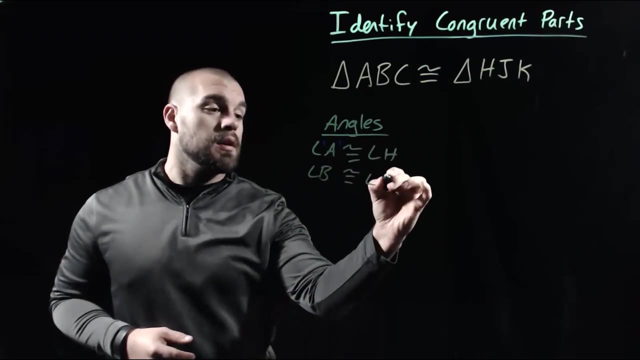 pieces in the same order. So if we look at angle A, from our first triangle, that has to be the congruent to angle H, because they're both in that first position when we're naming this thing. Then if we look at angle B, angle B came second and angle J comes second. So those two pieces have 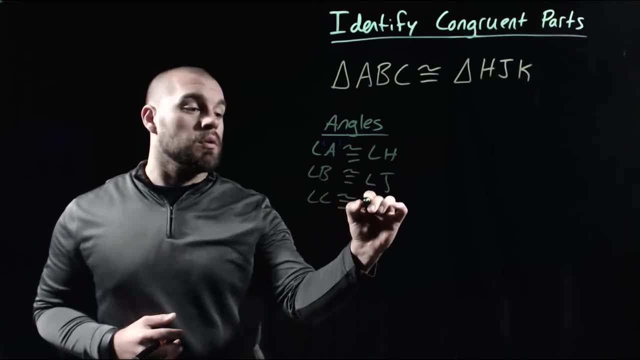 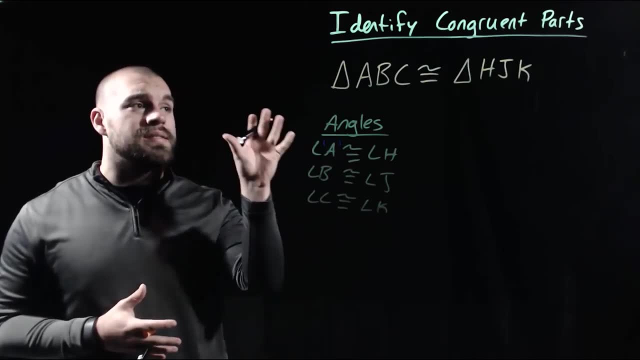 to be congruent, And then angle C is going to have to be congruent to angle K, because those things came third in the list. The sides might be a little trickier. So what I'm going to do is I'm going to use this congruent statement to draw out a picture.